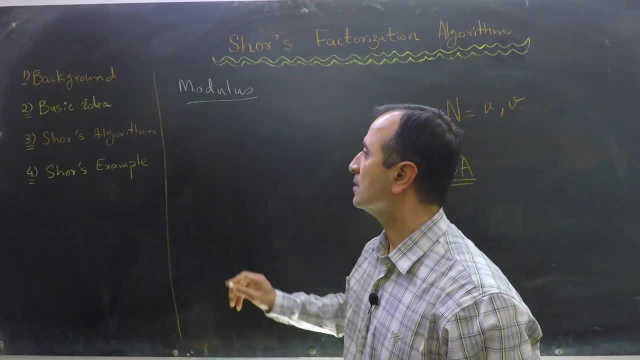 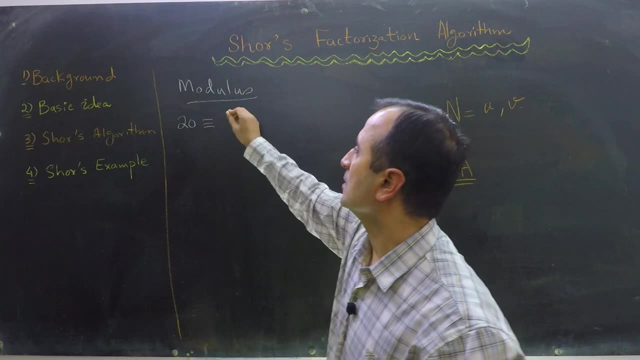 system And we will see that we already know the basis of the Shor algorithm. So here I will start from the initial function. So I have an initial function and the answer to this function is term of the Shor algorithm. So, as you can see, I have a number theory. And what is the value of this number theory? 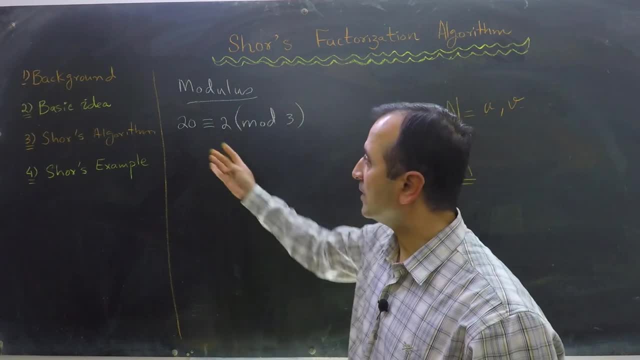 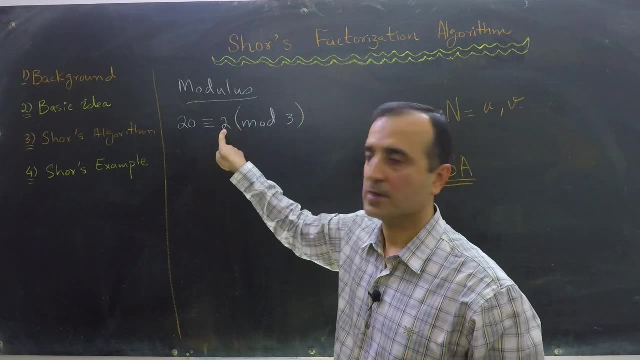 Well, the number theory is: 1 over Natorial 20 is same as 2.. It is because when we divide 20 from 3, our remainder is 2.. So sometimes we call modulus arithmetic as remainder arithmetic, because we're talking about remainder. So 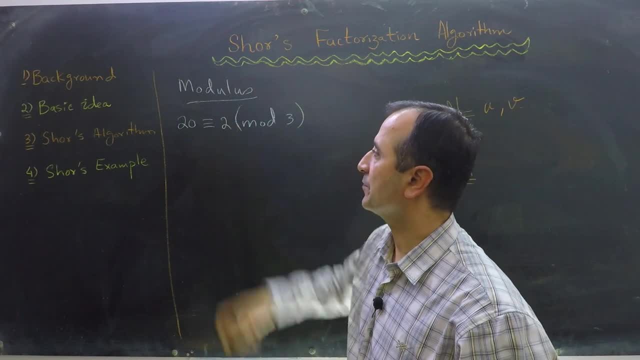 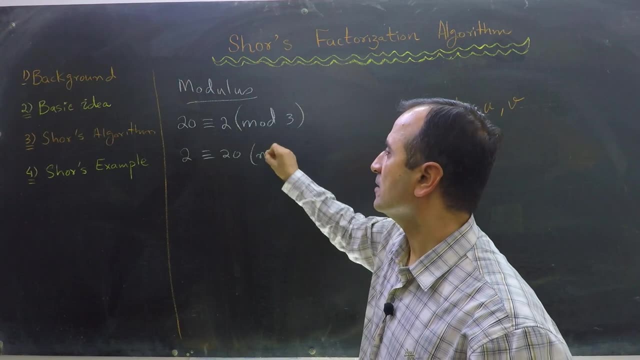 20 divided by 3, our remainder is 2.. Similarly, I can write it like: 2 is congruent to 20 in mod 3.. The reason I've written mod 3 in bracket is because mod 3 is with right-hand side as 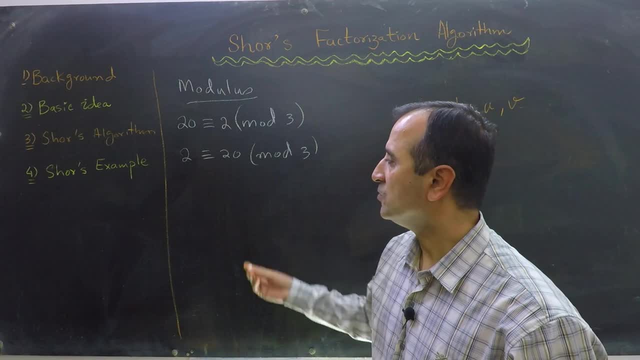 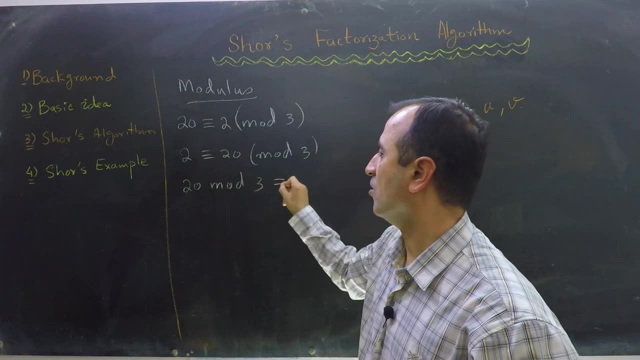 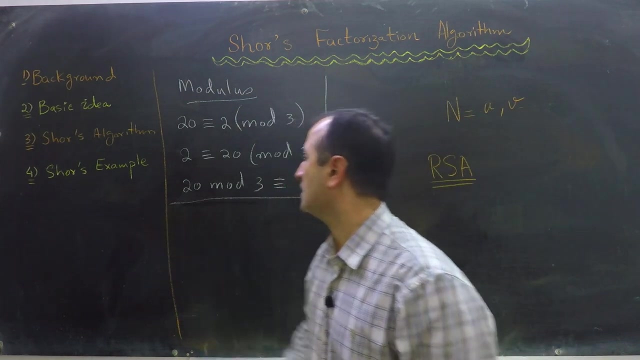 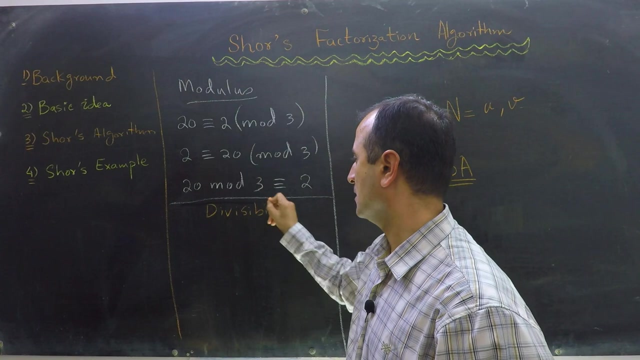 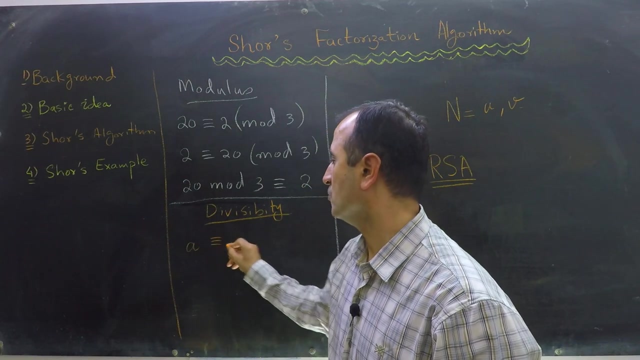 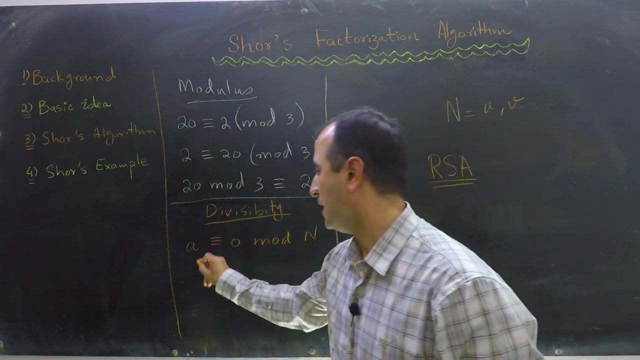 well as with the left long hand side. Similarly, I can also write this as: 20 mod 3 is congruent to 2.. Secondly, we must know about divisibility rules. So if I say that a is congruent to 0 in mod n, then it implies that n divides a. So let's do an example of this. 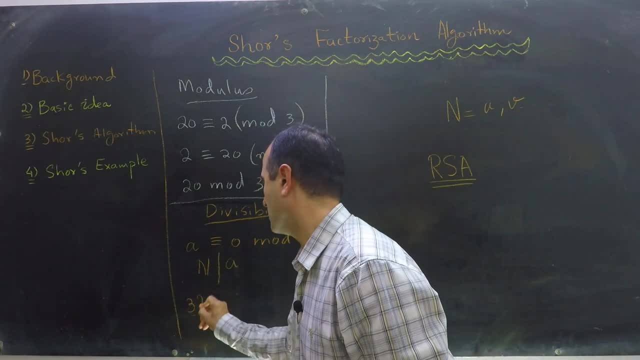 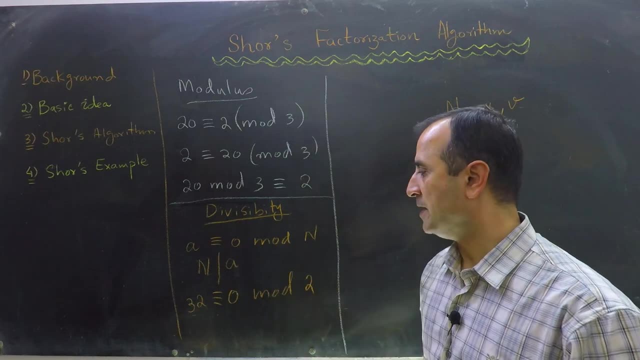 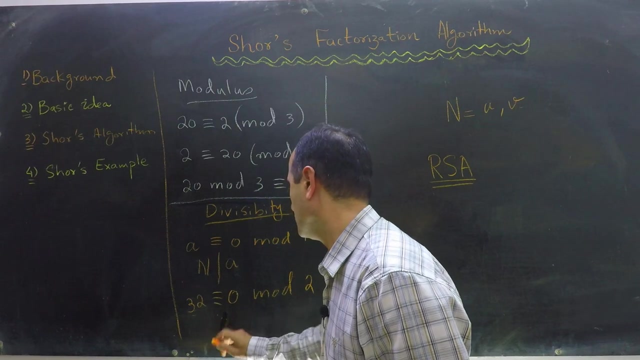 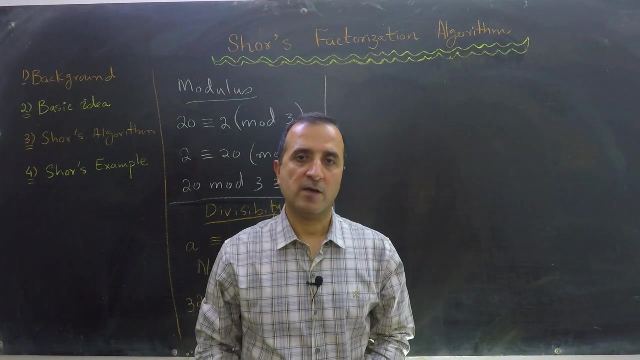 So I can say that 32 is congruent to 0 in mod 2.. That means if I divide 32 by 2, my remainder will be 0. Or I can say that 2 divides 32.. We should also be aware about. 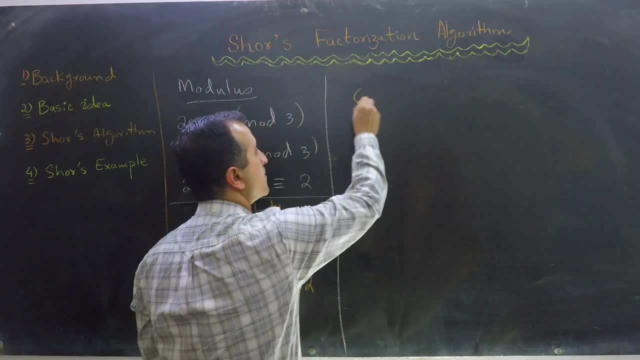 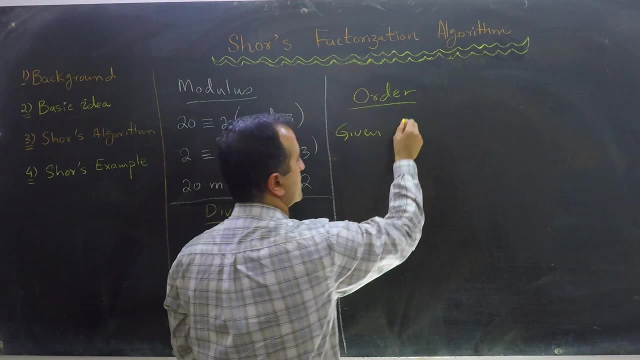 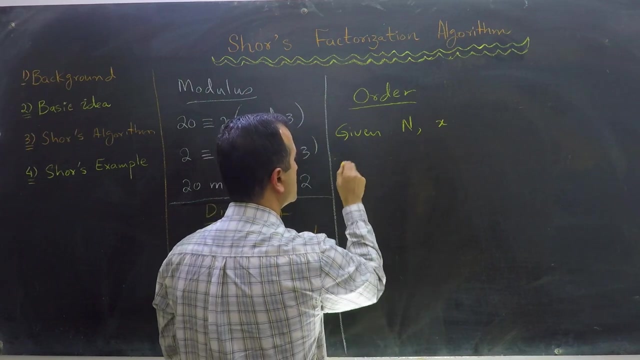 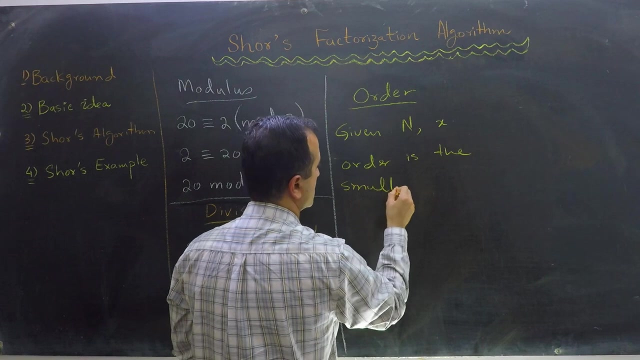 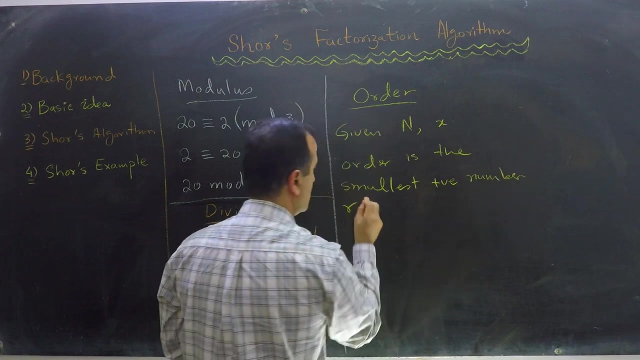 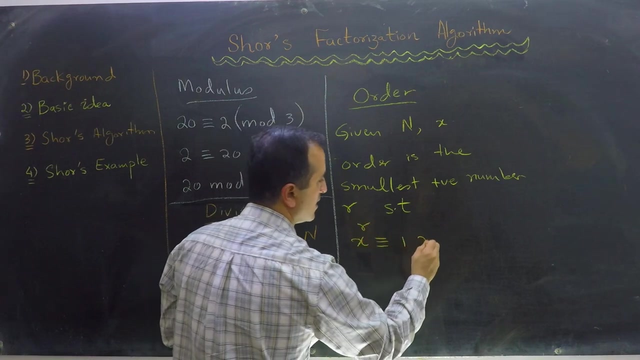 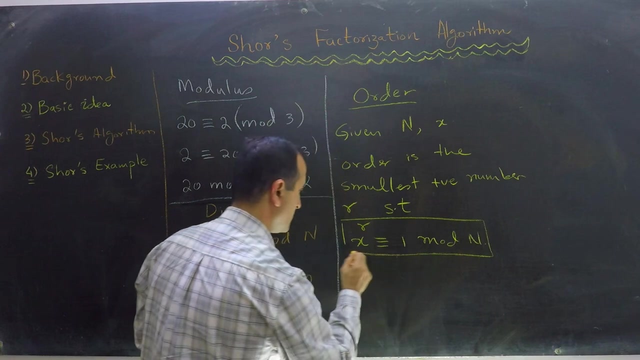 order of a group. So, given a number n and x, order of a group is a number r. Order is the smallest positive number, r, such that x raised to power r is congruent to 1 in mod n. Let's do an example of this. 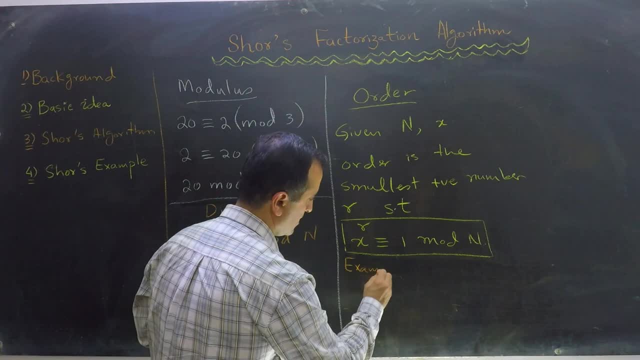 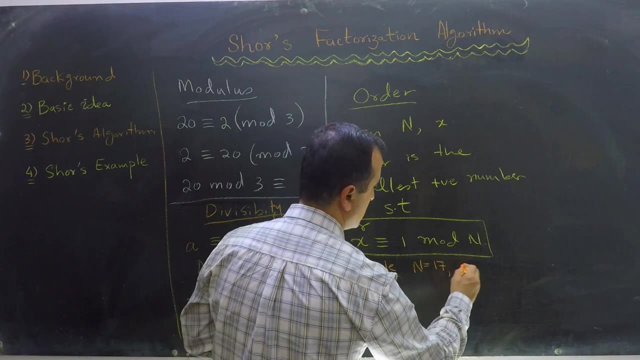 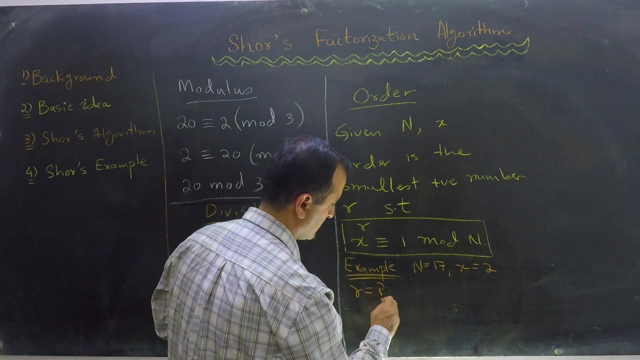 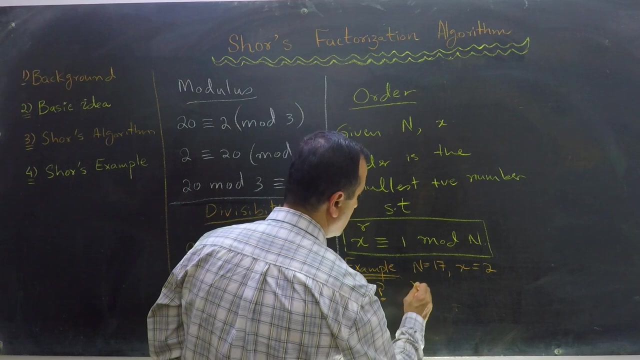 In this example, my n is 17,, my x is 2, and I have to find order r. So basically I have to use above equation. That means 2 raised to power r is congruent to 1 in mod 17.. 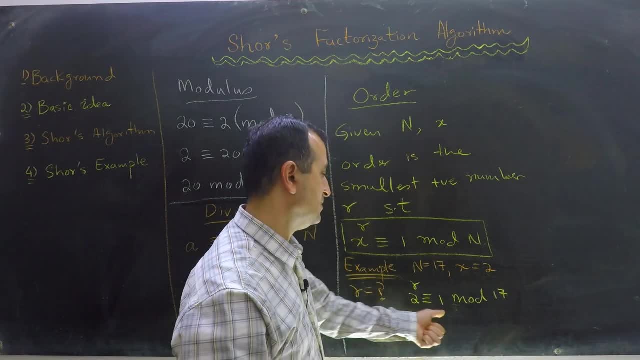 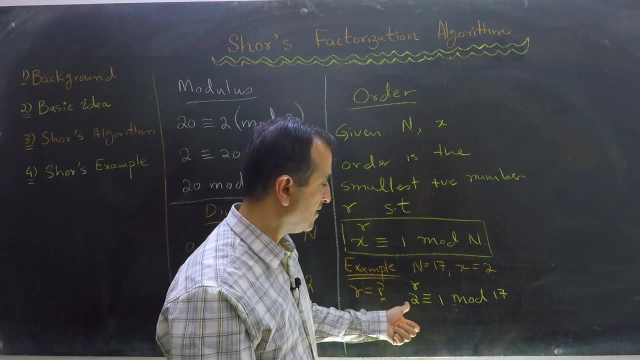 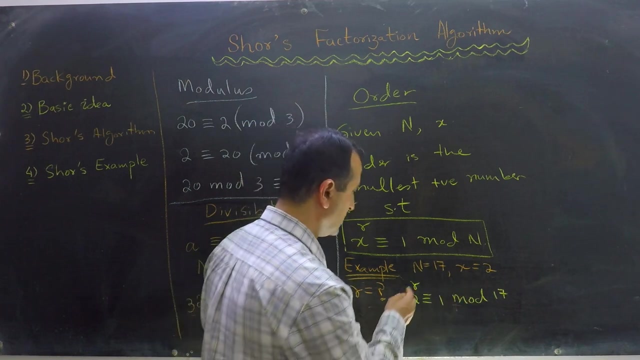 I will try different values of r, from 1,, 2,, 3, so on, such that for the smallest value of r, my 2 raised to power r, is congruent to 1 in mod 17.. After some calculation my r is equals to 8.. 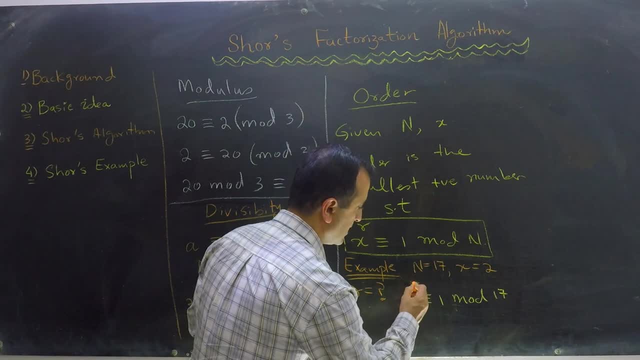 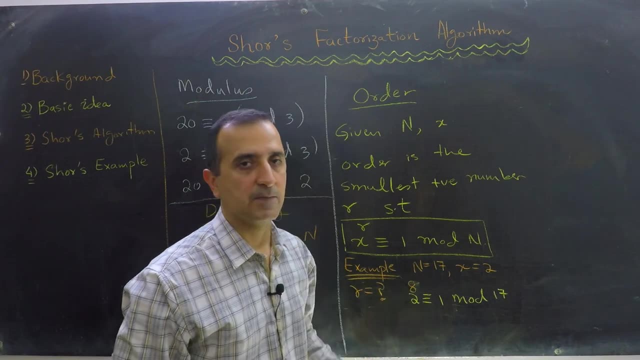 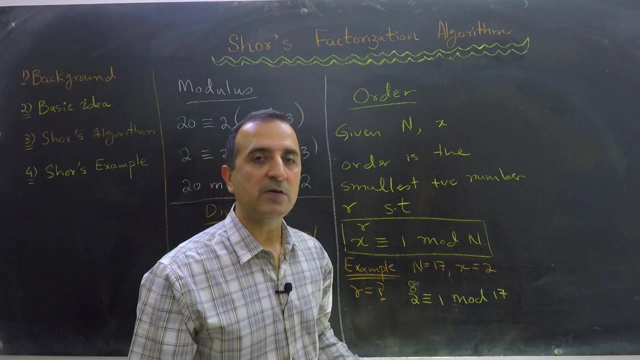 The algorithm of finding order on classical computer is exponential. But the algorithm of finding order on classical computer is exponential. But we will be using a quantum algorithm to find order And that algorithm I will explain in theory in the next video. We are done with our background. We have learned the basic mathematics that is needed to understand. 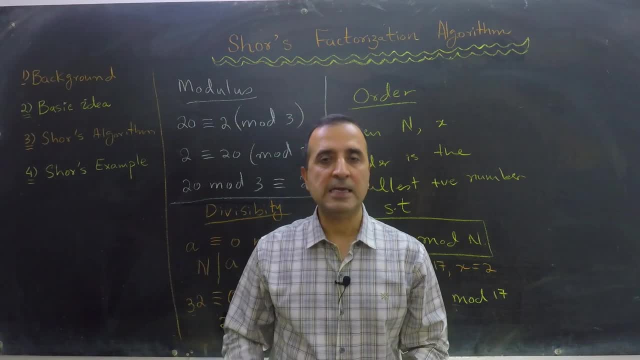 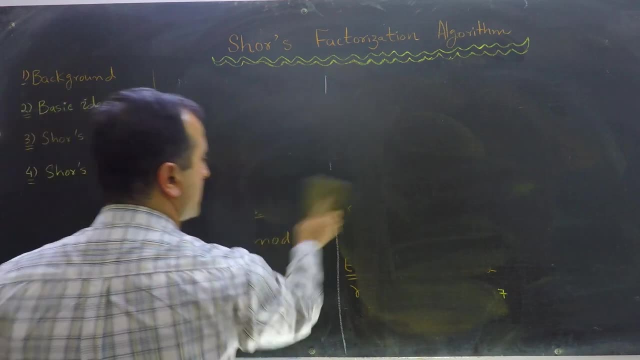 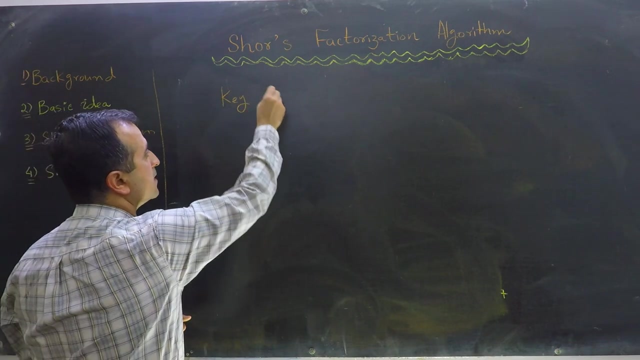 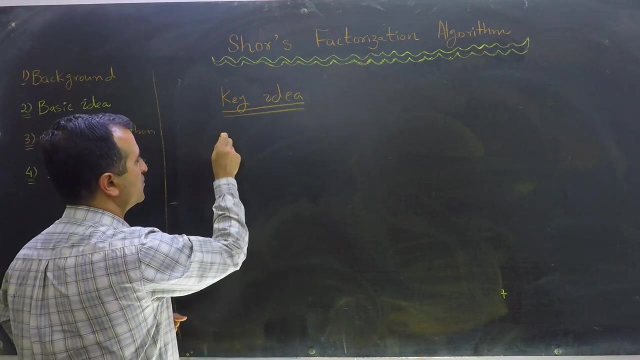 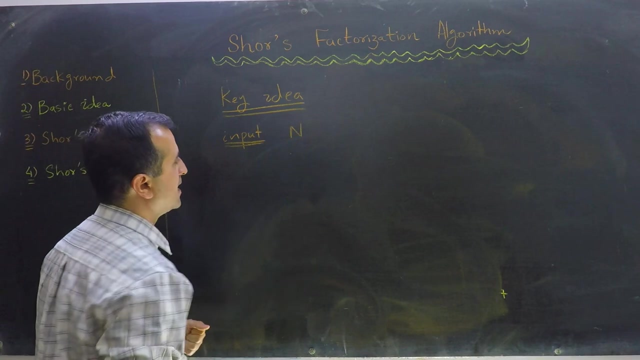 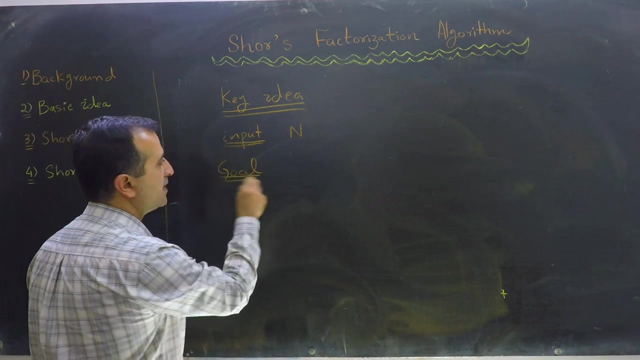 Shor. Now we will try to learn the key idea behind Shor algorithm. So our key idea of shore algorithm: Recall that for the shore algorithm our input is a composite number, n, and n is composed of two primes, u and v. Our goal is to find u and v. 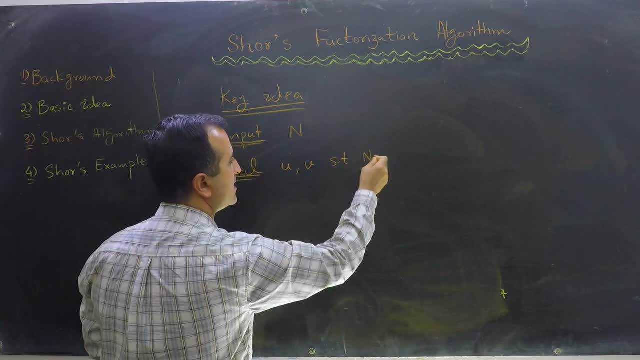 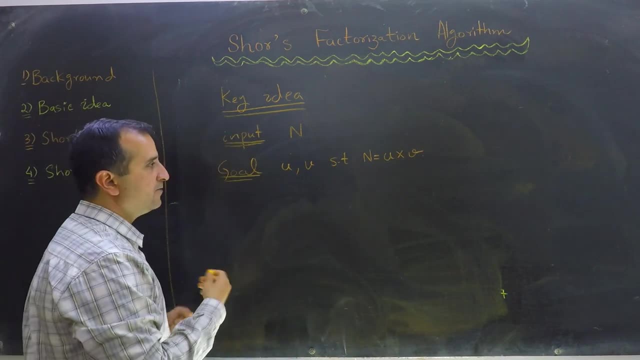 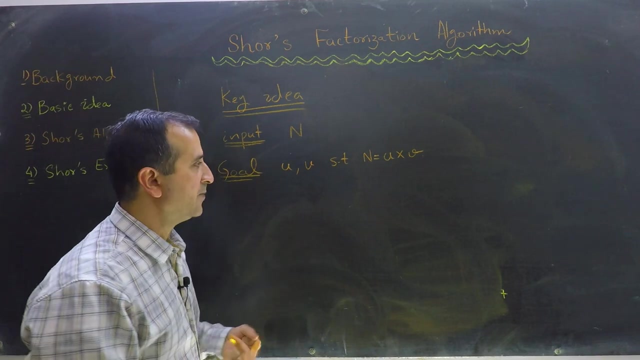 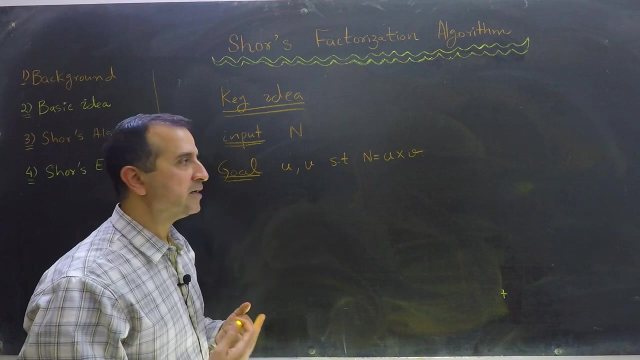 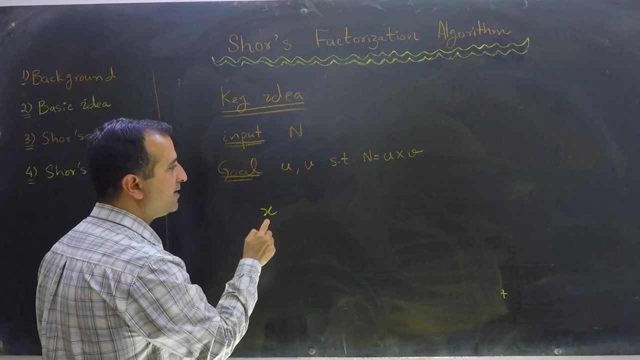 such that n is equal to u times v. So what shore algorithms do is that use order finding algorithm as a subroutine. So shore algorithm by itself is a classical algorithm, algorithm based upon simple number theory. but it calls order finding algorithm to find order which find order in polynomial time. So it takes a random x and for that random. 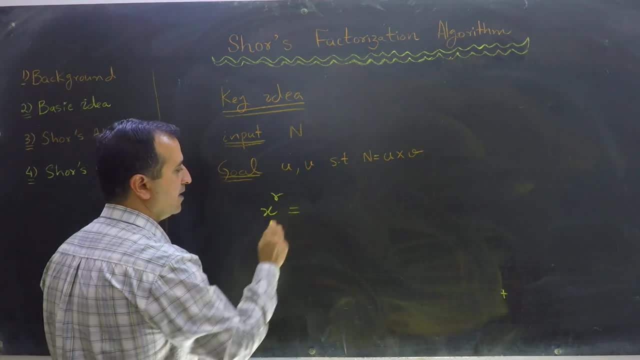 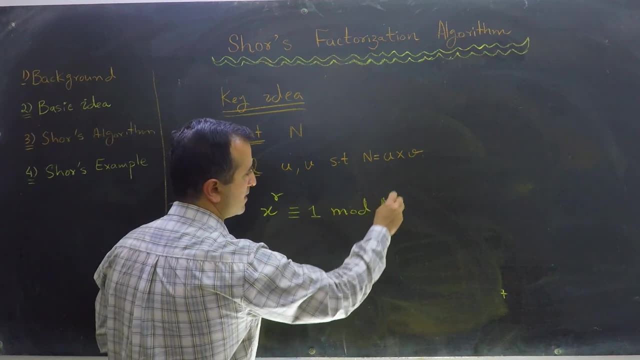 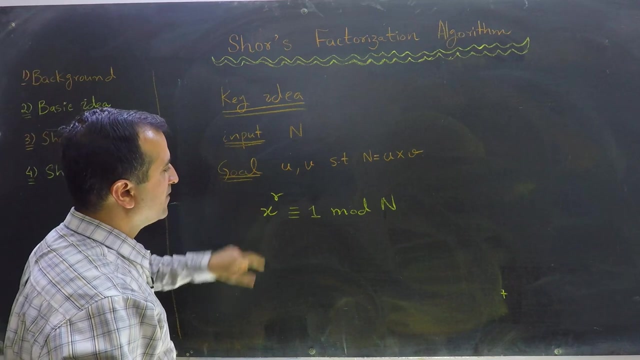 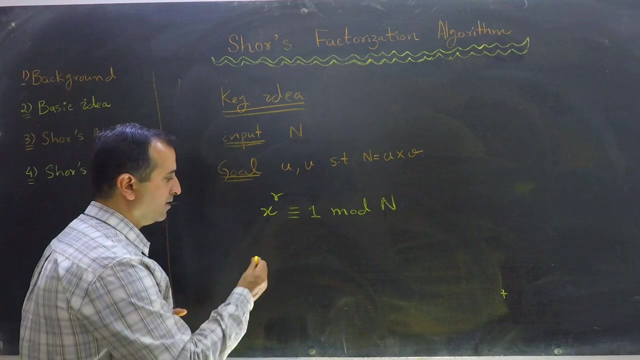 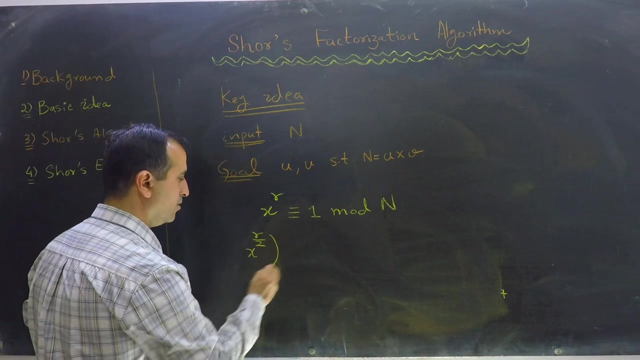 x. it finds order r such that x raised to power r is congruent to 1 in mode n. This n is our input, our composite number, And then it checks if our r is even or odd. If our r is even, then I can write this equation as x raised to power r over 2 whole square. 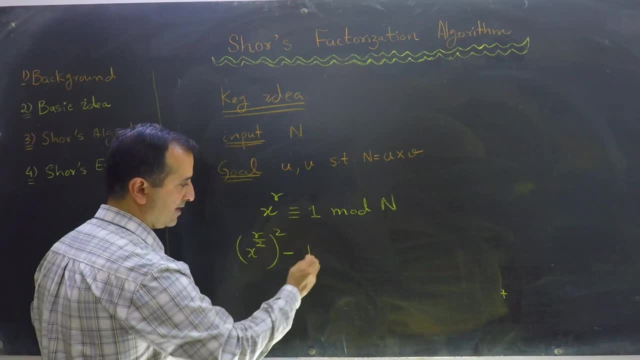 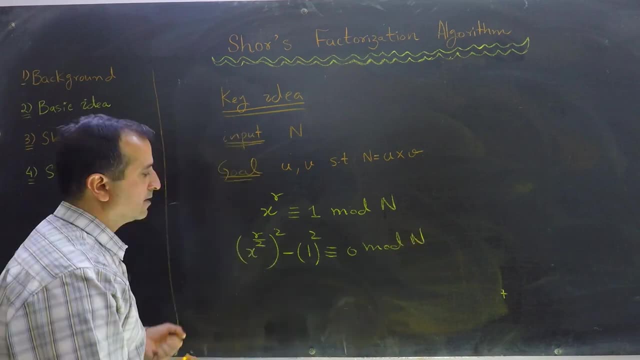 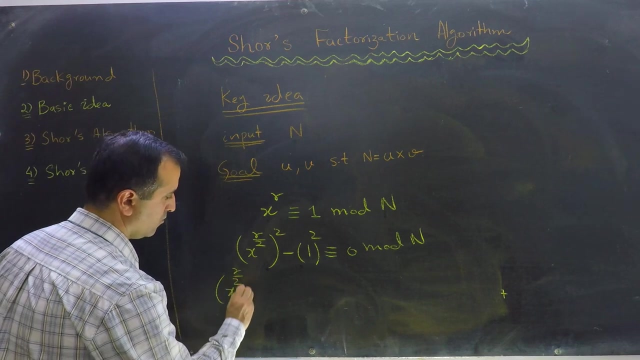 minus. I take this 1 to this side minus 1 whole square is congruent to 0 in mode n. Then I can just expand this So it will become x r over 2 minus 1 times x r over 2 plus 1. 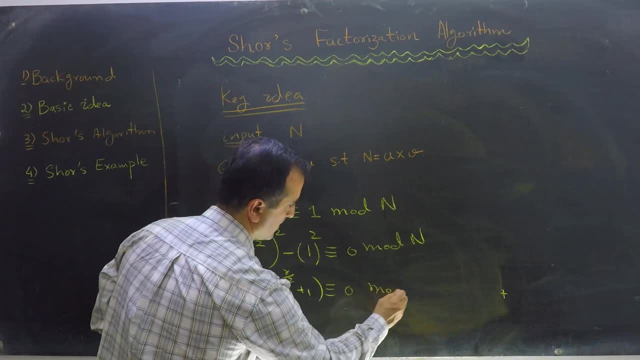 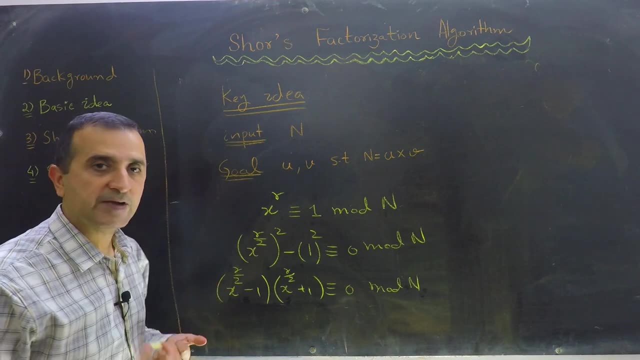 is congruent to 0 in mode n, This square root of x will be either trivial or non-trivial. By trivial it means that x raised to power r over 2 is congruent to 0 in mode n. So this square root of x will be either trivial or non-trivial. By trivial it means that: 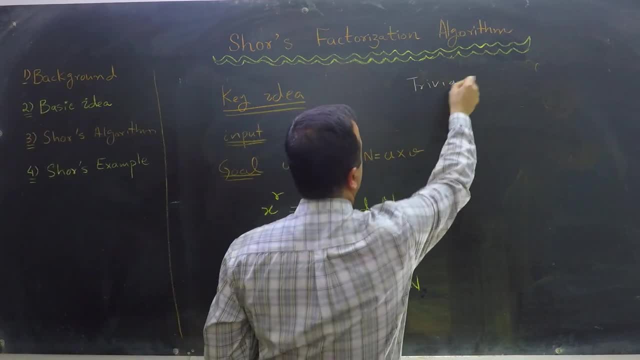 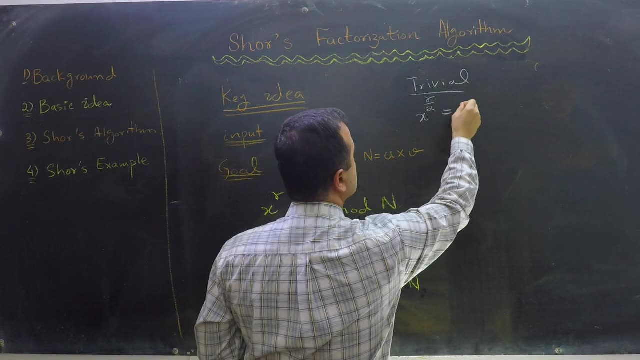 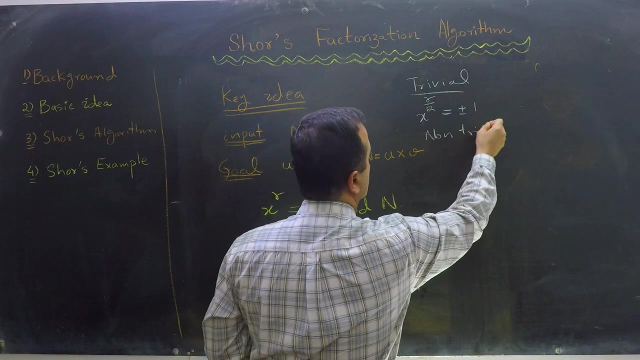 x raised to power r over 2 is congruent to 0 in mode n. So this square root of x will be either trivial or non-trivial, And in case of non-trivial it implies that x raised to power r over 2 will be equal to plus minus 1.. And in case of non-trivial x raised to 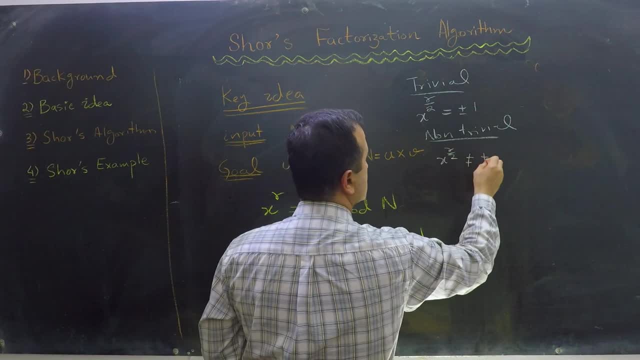 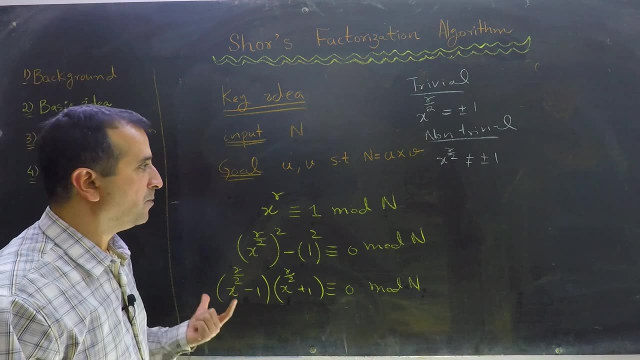 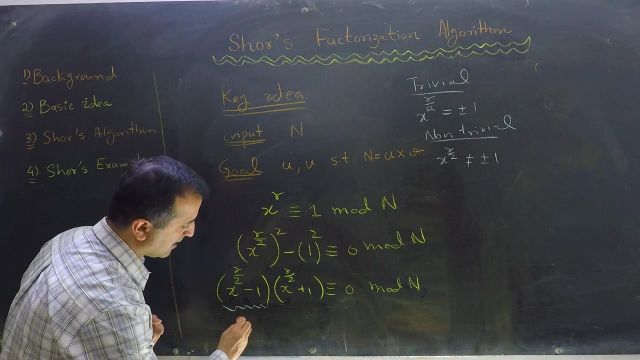 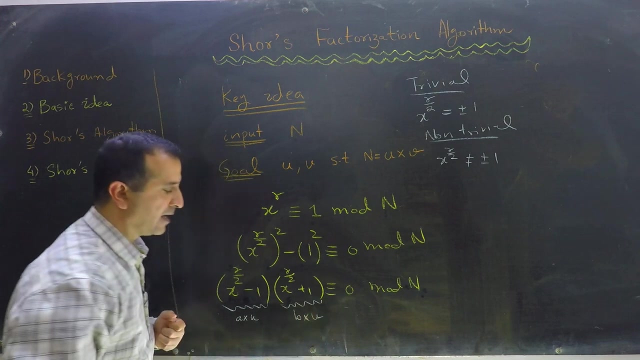 power r over 2 will not be equal to plus minus 1.. If these square roots are non-trivial, then they will be equal to 0.. multiple of u and v: That means this might be a times u and this might be b times v. 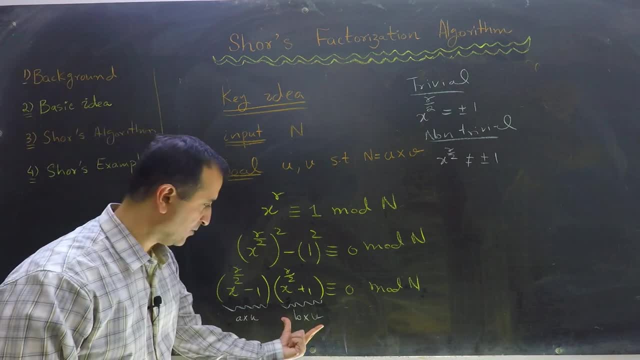 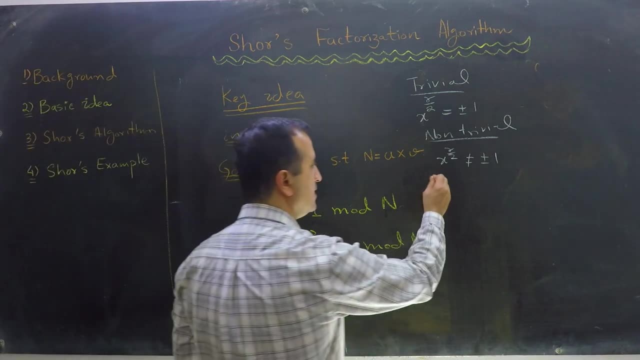 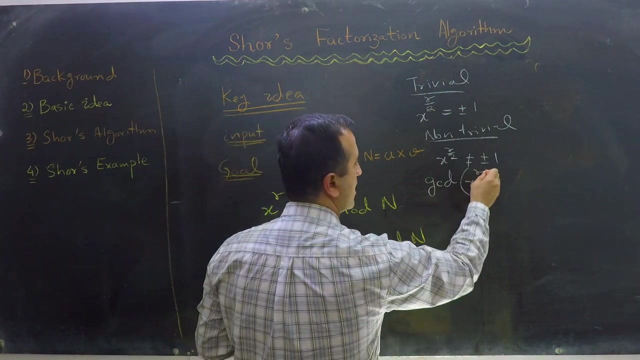 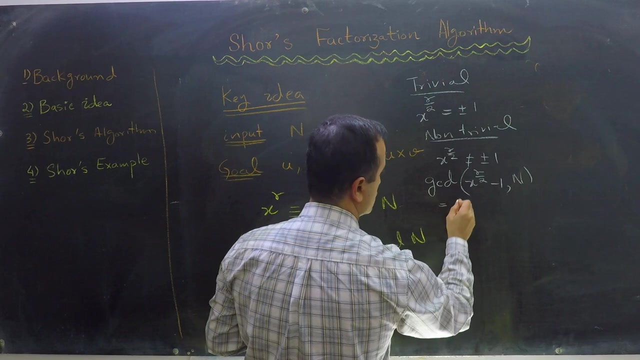 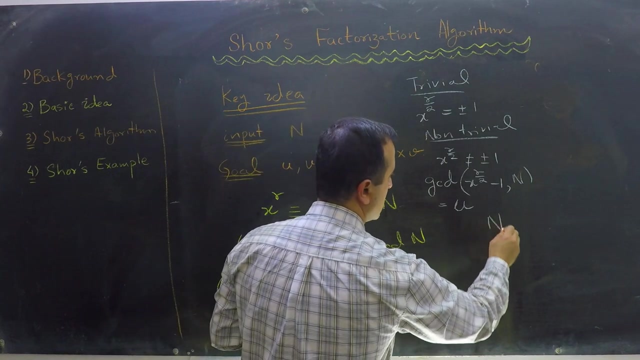 In order to retrieve u from this or v from this, we can take GCD of this with n. So GCD of x raised to power r over 2 minus 1 comma. n will give me u And then to find v, I simply divide n by u and that will be my v. 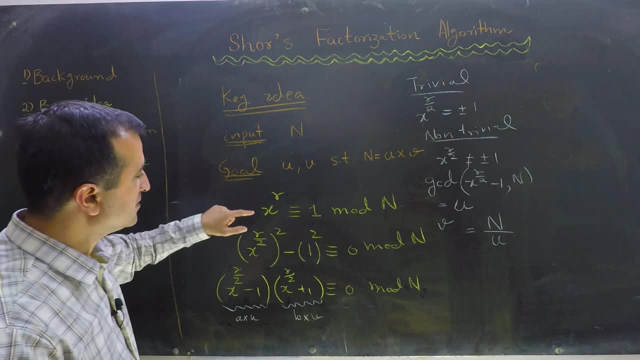 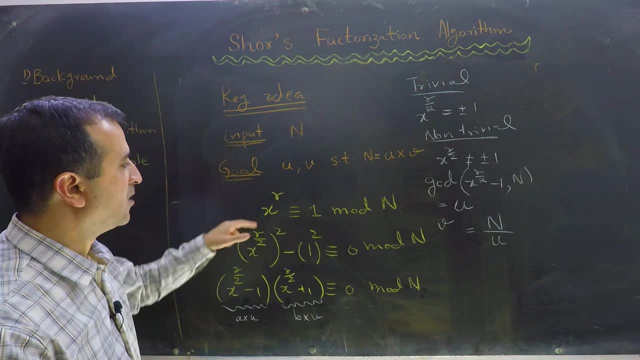 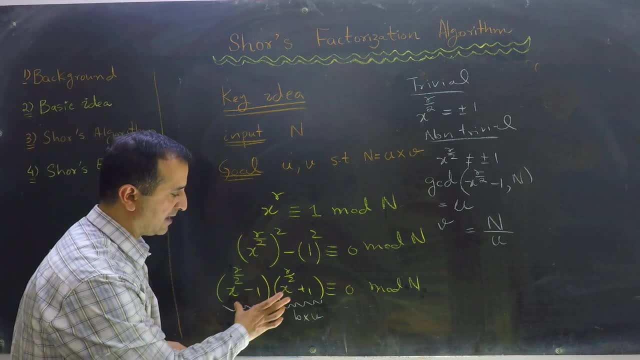 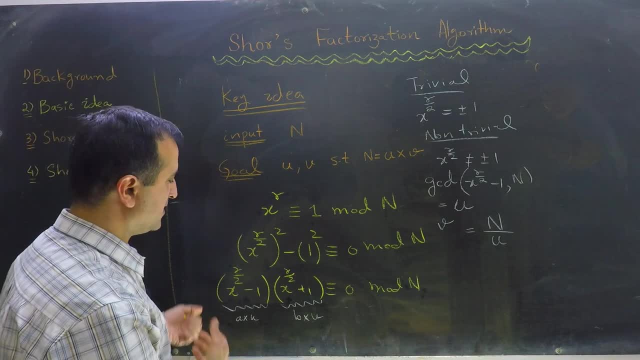 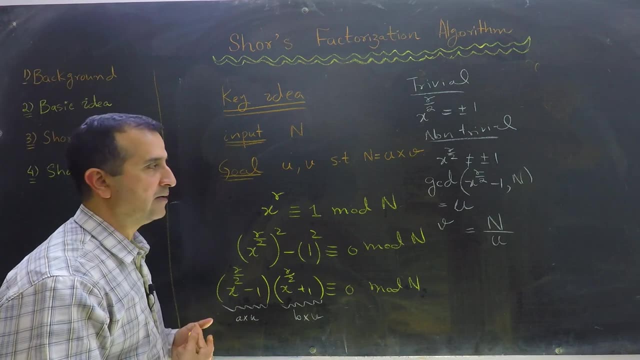 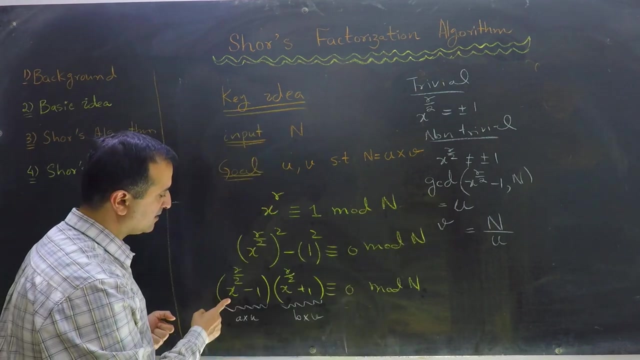 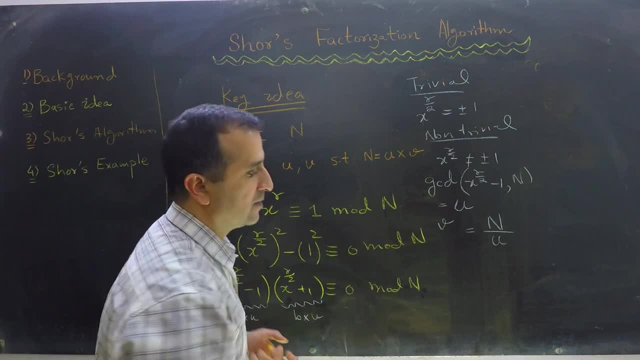 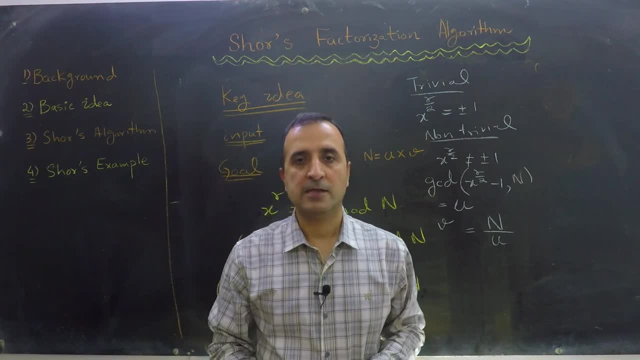 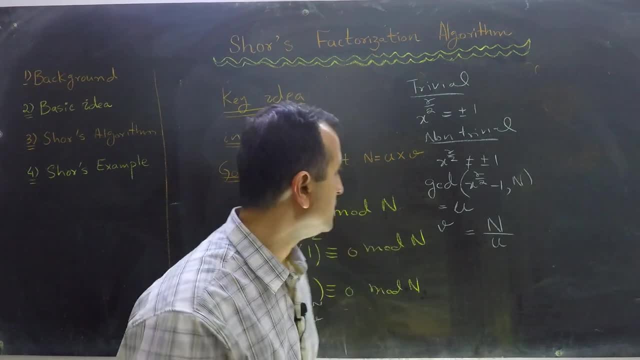 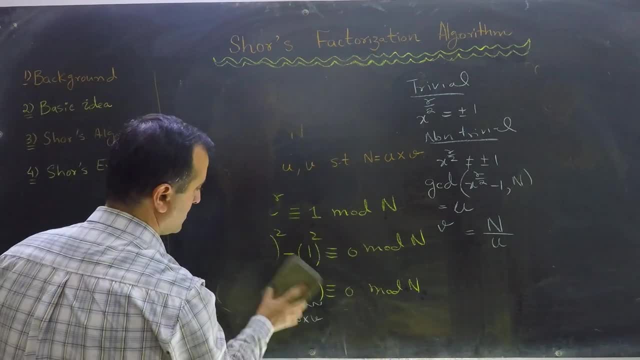 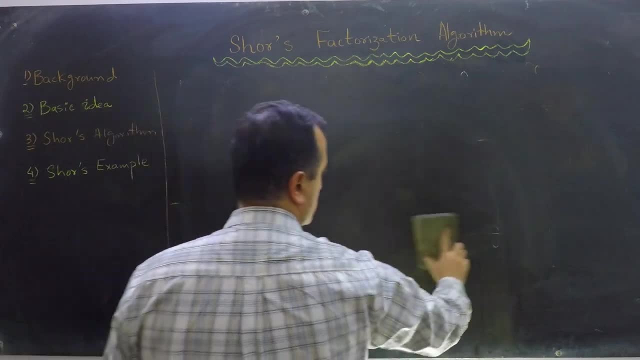 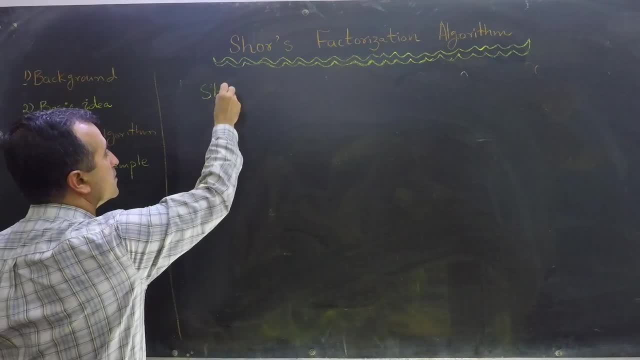 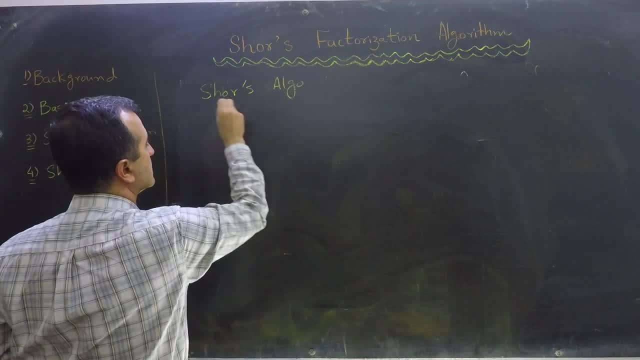 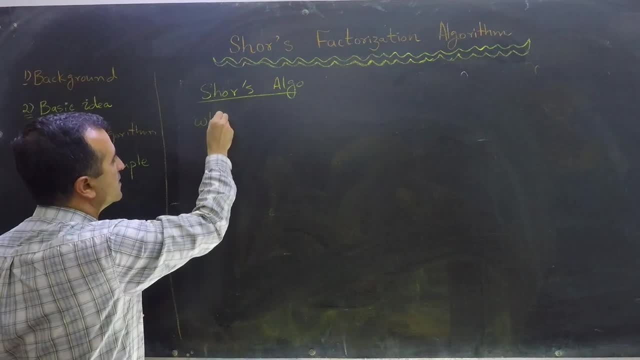 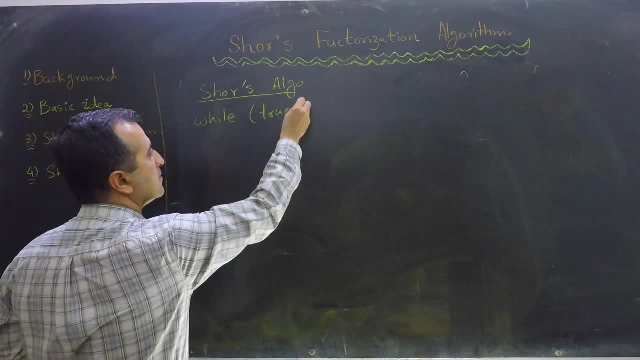 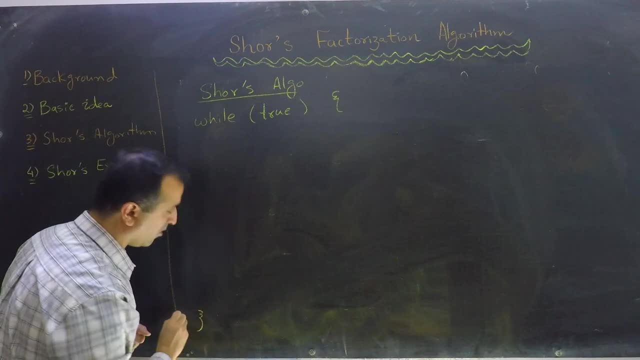 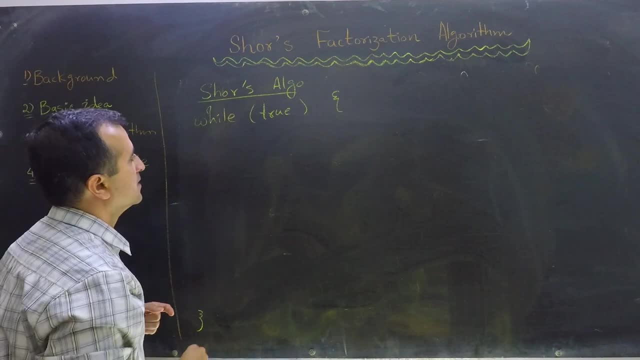 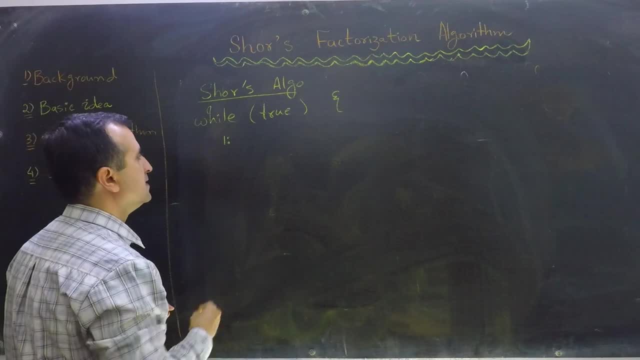 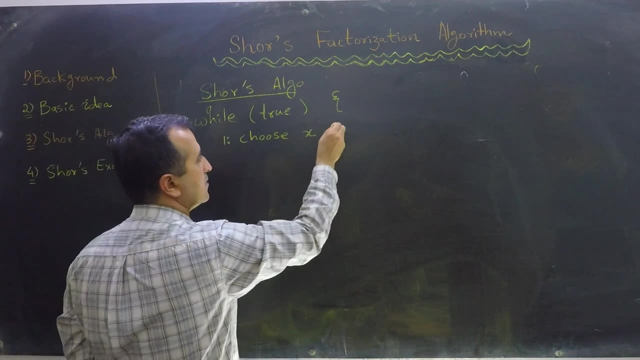 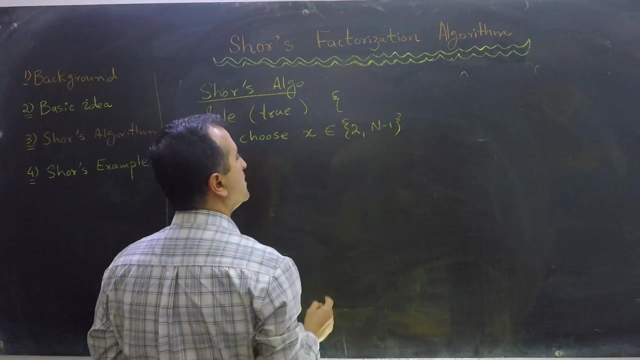 So, in short, I have to first find v. So, in short, I have to first find v. So, in short, I have to first find v. that we choose randomly x from 2 to n minus 1.. n is our input. We want to. 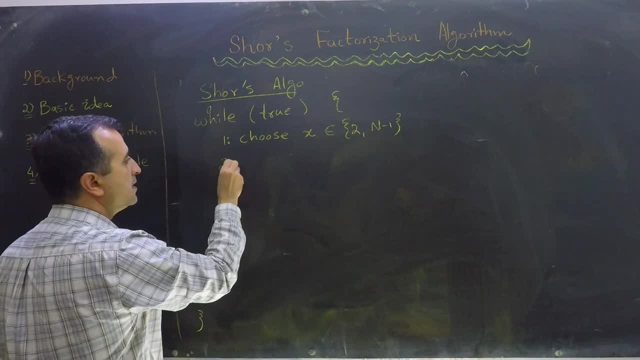 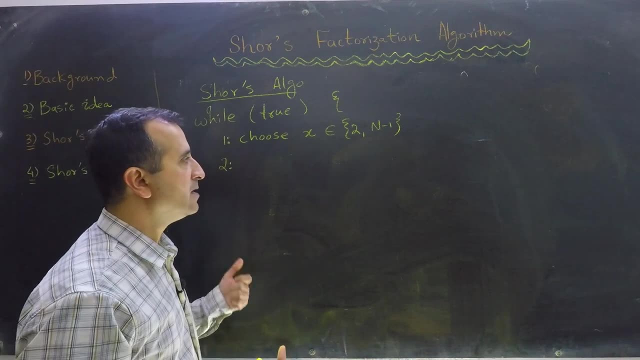 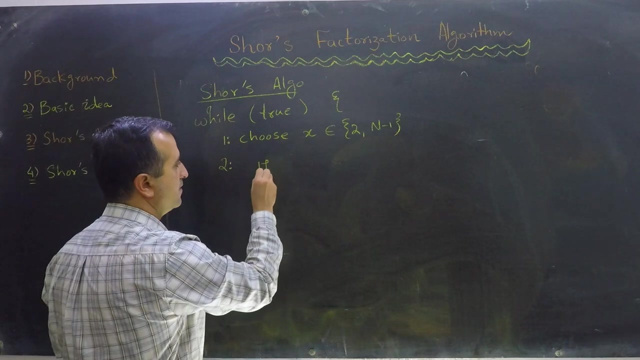 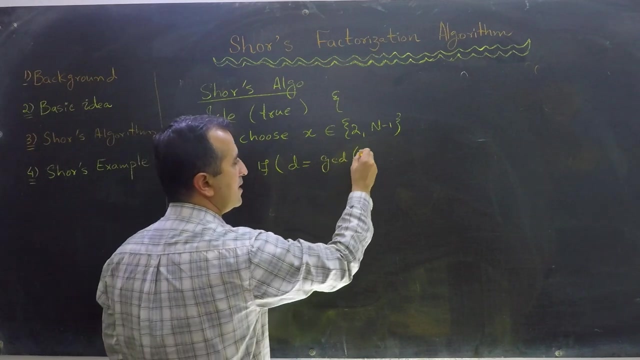 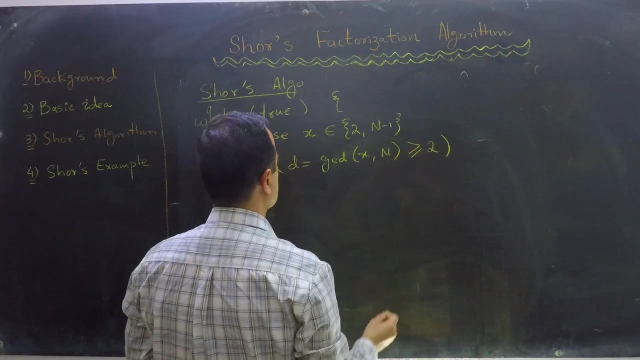 factorize n, Step 2.. Now, in very rare case, in one in trillion chances, we could be extremely lucky and x could be our factor of n. So let's check that If d equals to gcd of x, comma n is greater than equals to 2, then this is the case. 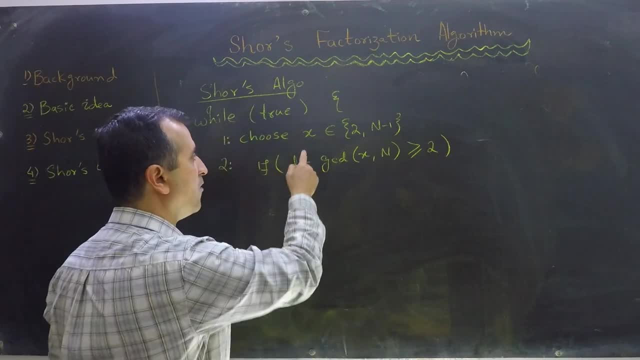 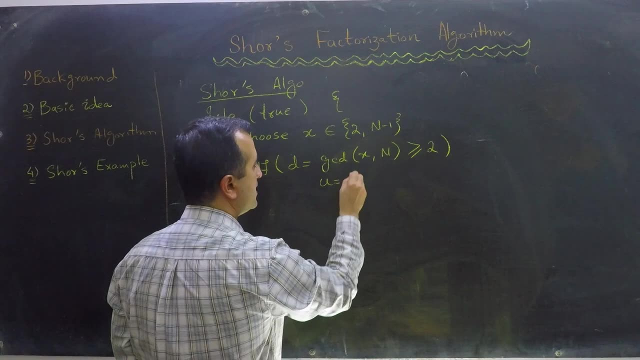 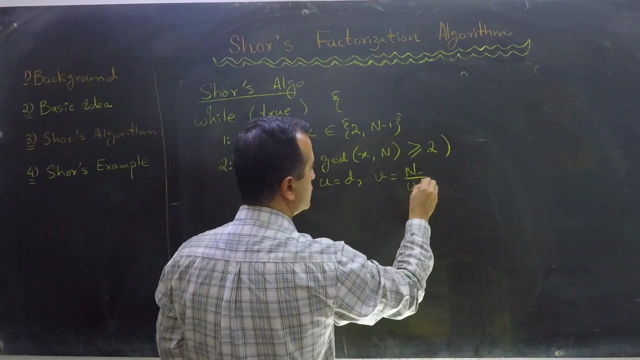 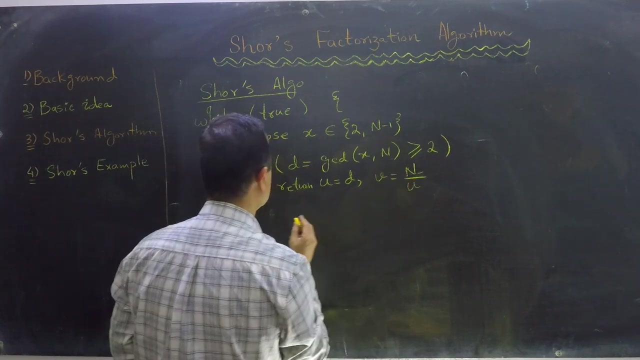 that we are extremely lucky and by some chance we have found a factor of x by luck. So we just say that u will be equals to d because we have found a factor, and v will be equals to n over u and we return our u and v. So this is the. 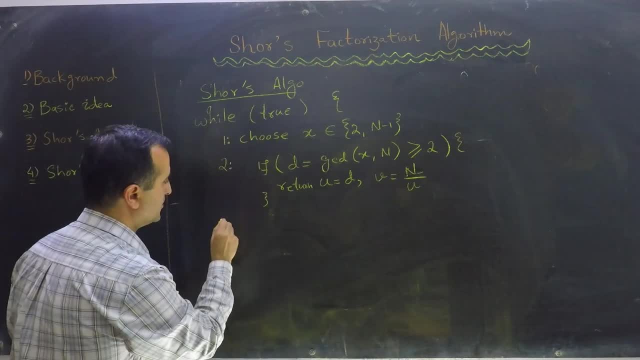 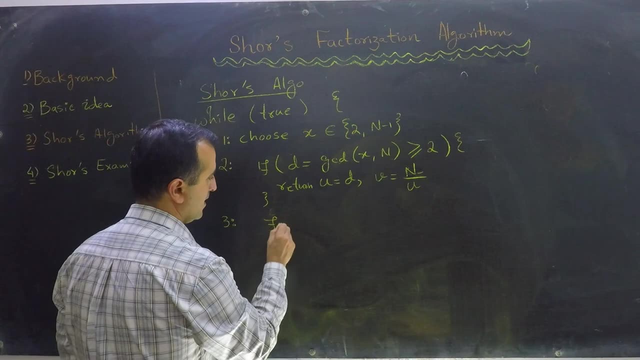 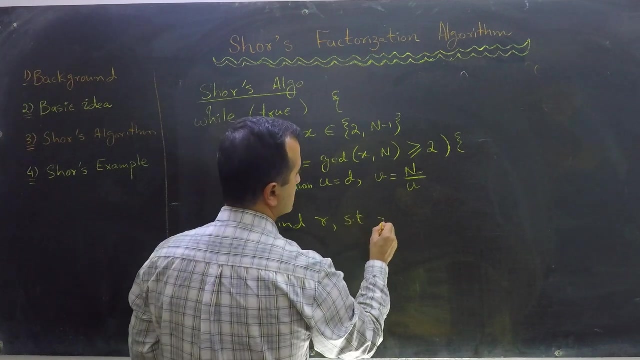 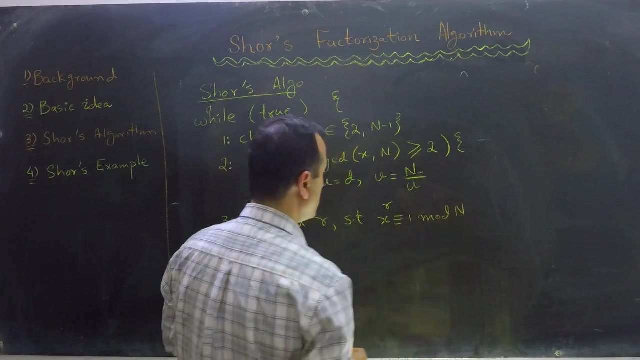 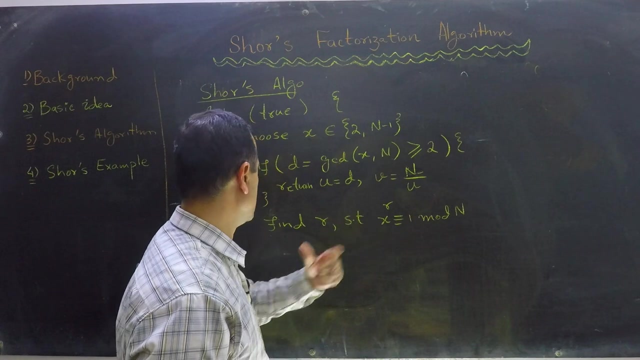 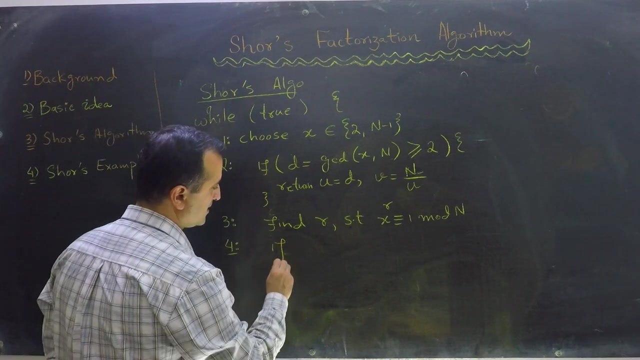 end of our if condition, Step 3.. Otherwise we will find r such that x raised to power, r is congruent to 1 in mod n. Here we are calling our quantum subroutine of order finding algorithm. This will be the subject of next video, Step 4.. Now we have if condition. 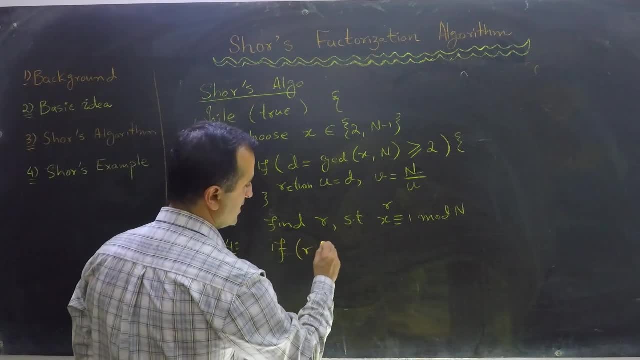 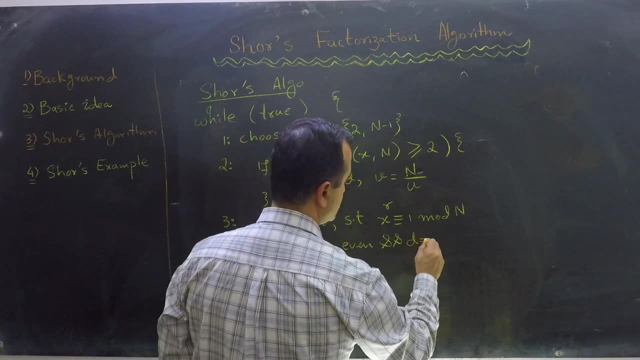 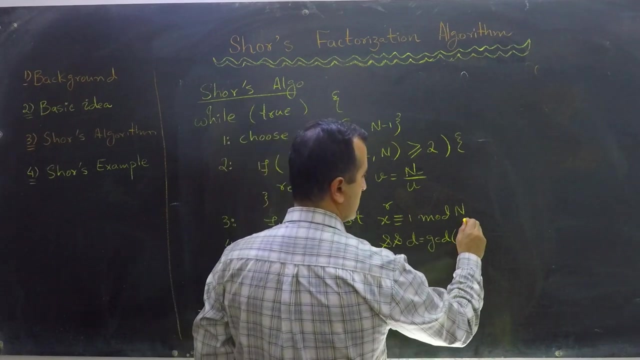 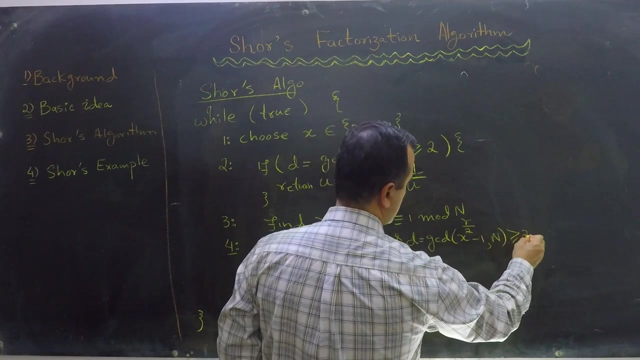 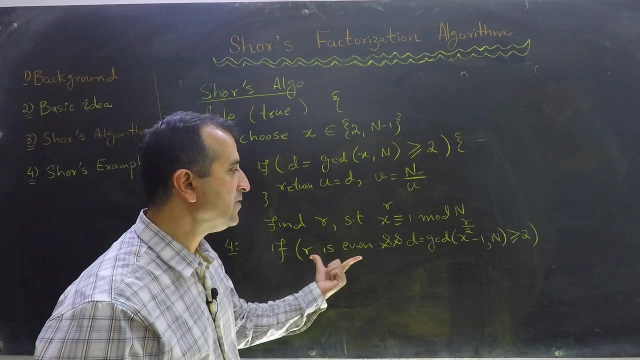 if r is even and d equals to gcd of x raised to power r over 2 minus 1 comma, n is greater than equals to 2.. So the first condition is checking that our order is even, and, And when our order is even, then we are checking the second condition. 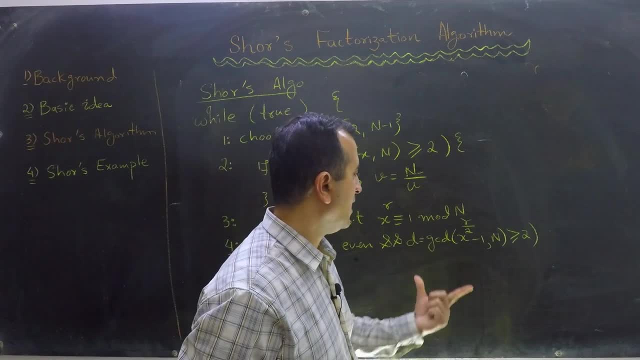 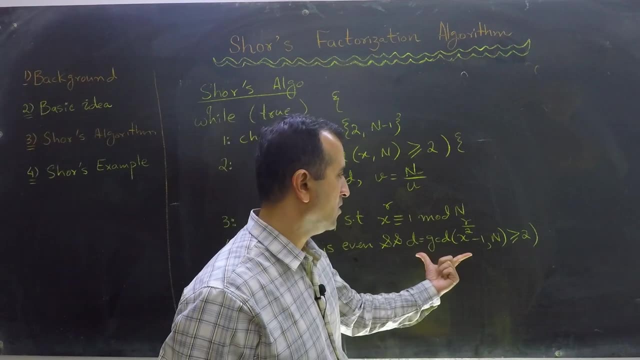 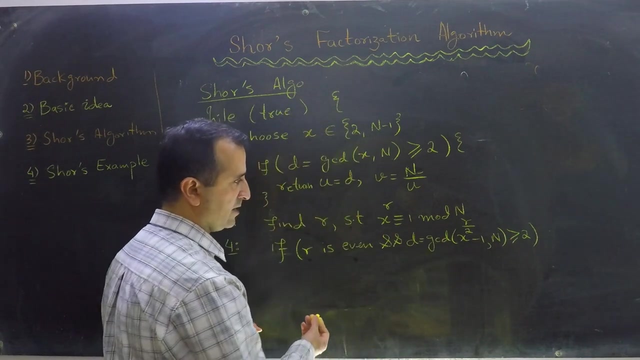 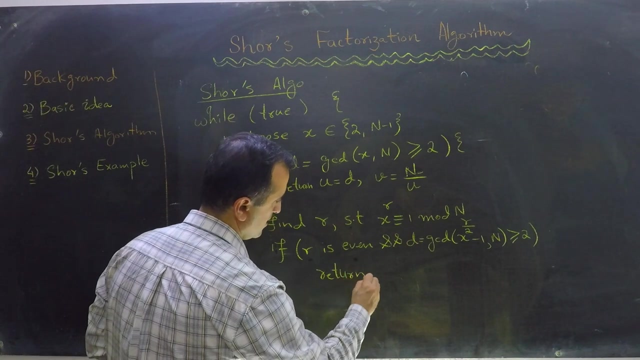 In the second condition we are checking if our square root of r is trivial or not, Because if our square root of r is non-trivial, only then our GCT will be greater than equals to 2. When our square root is non-trivial and r is even, then we once again return u equals. 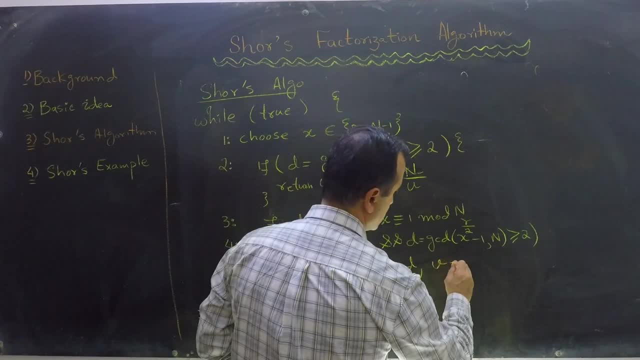 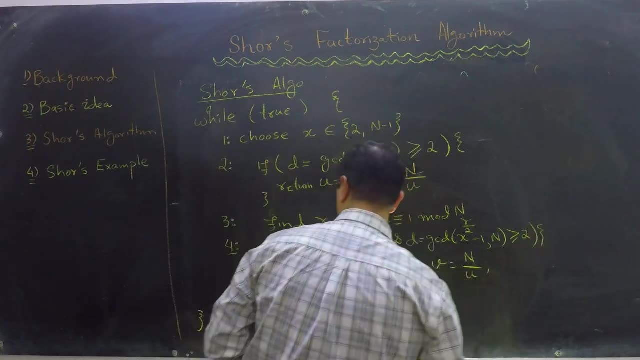 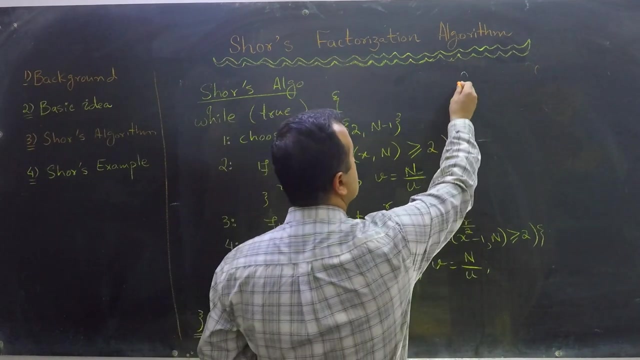 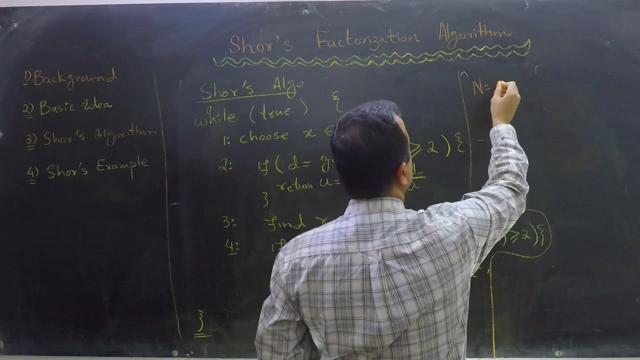 to d and we return v equals to n over u. So that is the end of our algorithm. Now let's do an example to make it even more clear. In this example, my n is 221.. I have to find factors of 221. 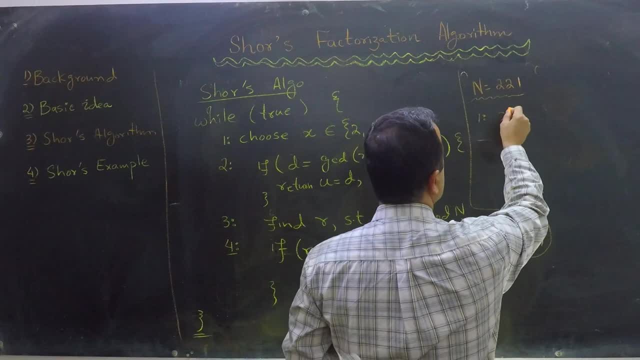 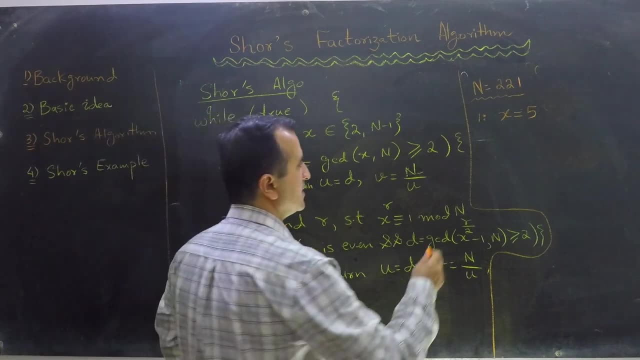 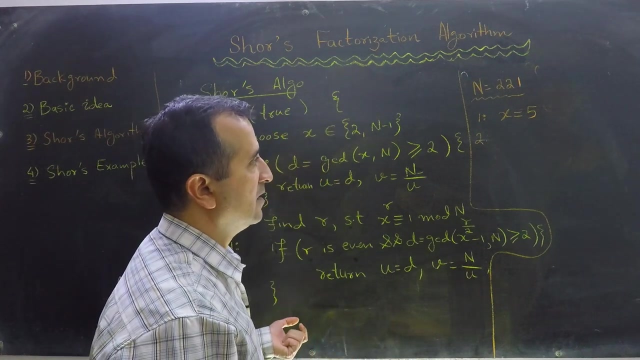 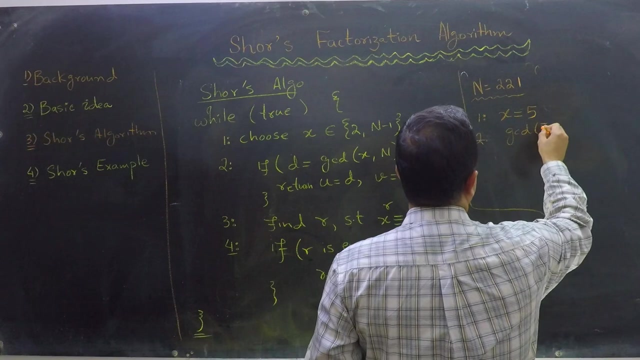 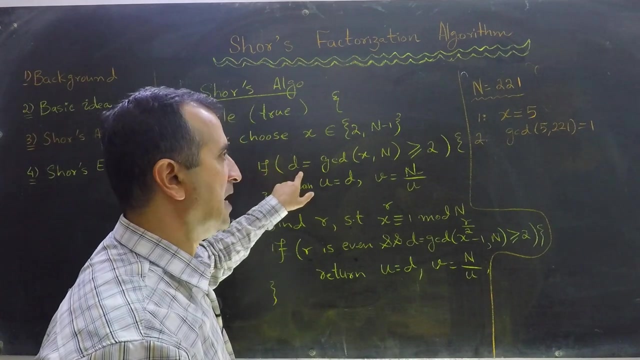 I do my first step. my x is equal to 5.. Now I do my second step, that I check if x is by any chance a factor of n and gcd of 5 and 221 is equals to 1. That means this: if condition will be false and I am not lucky, 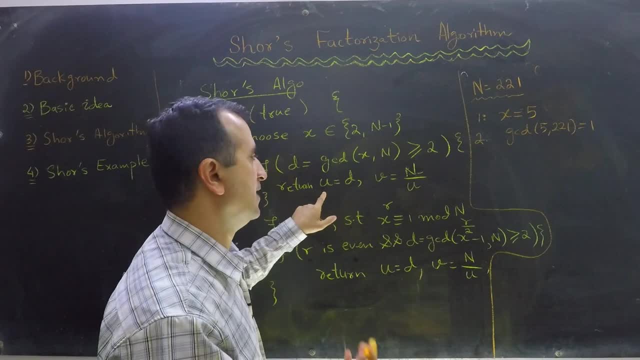 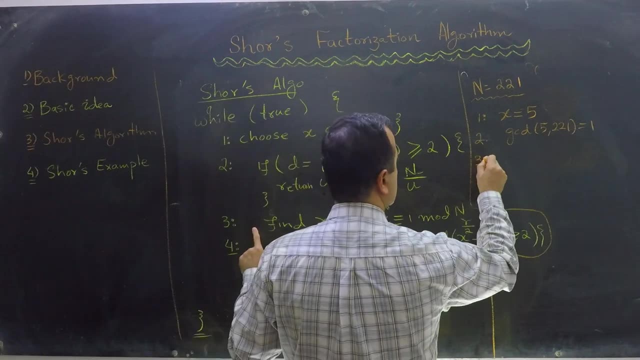 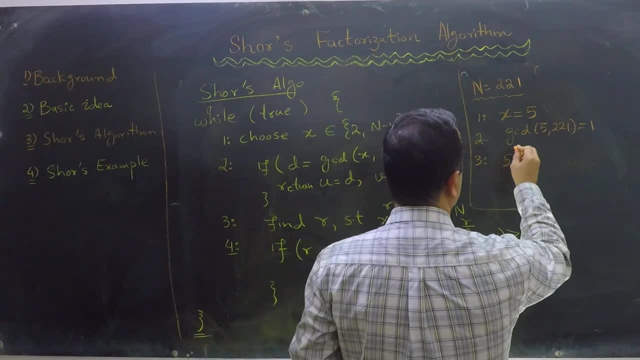 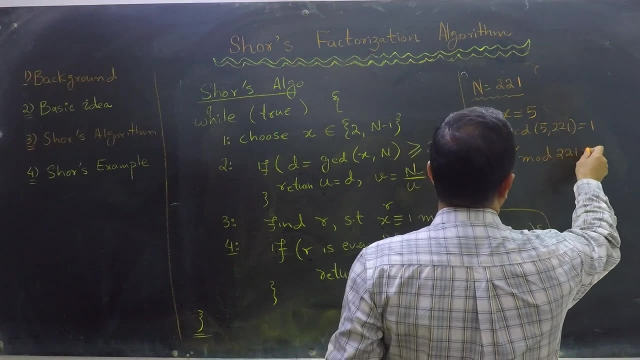